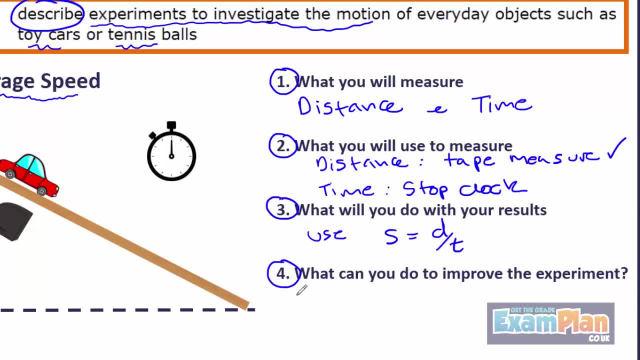 equals distance. We will now calculate the time measured instead of the estimated time measured by our results. As you can see, the average value is now one metre. Let us now go back and look at our results. To improve our investigation, we can repeat the measurements, not only take an average. 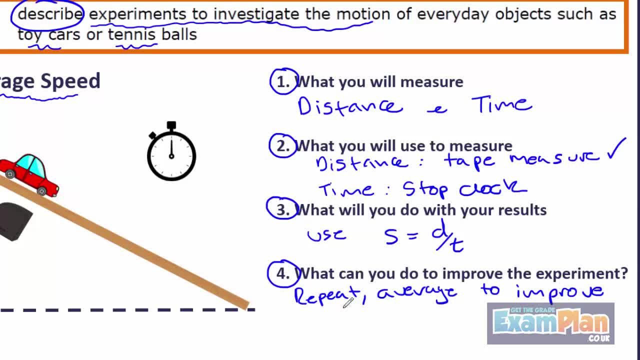 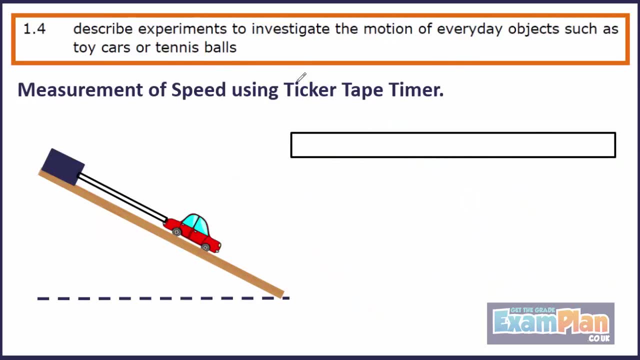 but also take a repeat. It is important to say that we are going to take an average and why we are doing this, ie to improve our reliability. simply stating that to take repeats is not sufficient In this investigation. we will also look at measurements Well, to make these investigations. 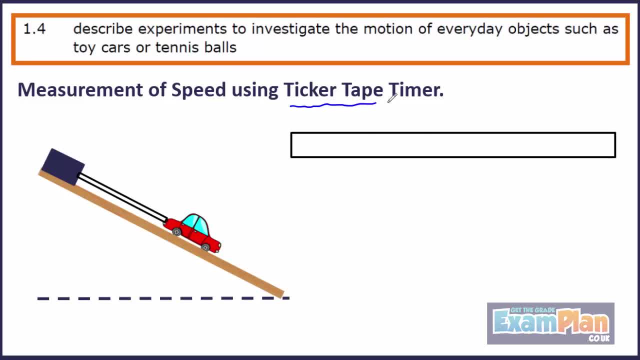 we need to have a baseline so that we can calculate the times measured by our results. Of course, if you want to do this, you can also take a look at the measurements we show on our website measuring speed, but this time we're going to use a ticker tape. A ticker tape is a thin 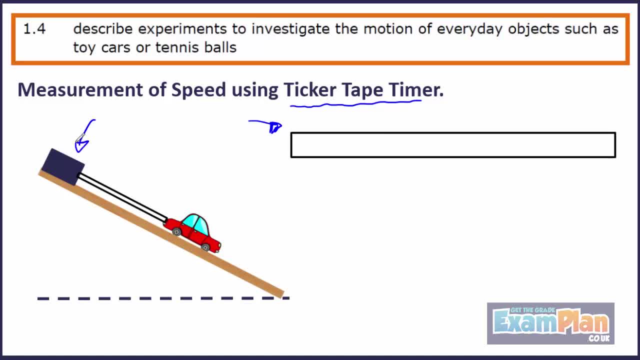 strip of paper that passes through a ticker tape machine. We attach the ticker tape to the back of the trolley and feed it through the machine. The machine then punches dots on the paper every 0.2 seconds. So if we know the distance between a set of dots and we, 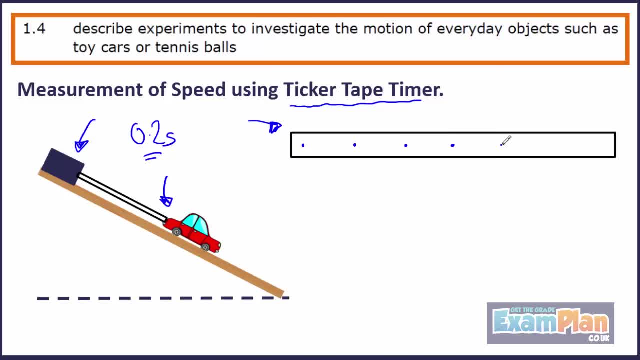 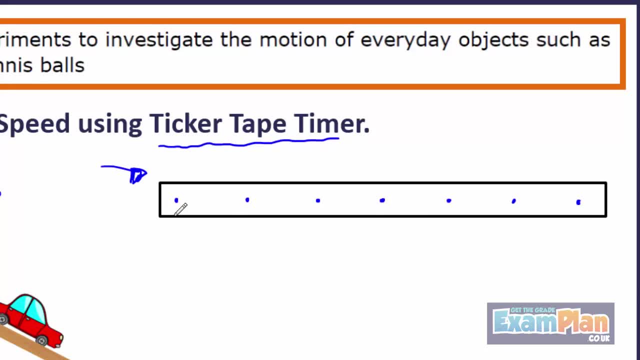 know the total time, we can work out the speed. So let's look at an example. Imagine we have a ticker tape with dots evenly spread. This tells us the car is going at a constant speed. but more on that later We can pick a pair of dots. the further apart the better. 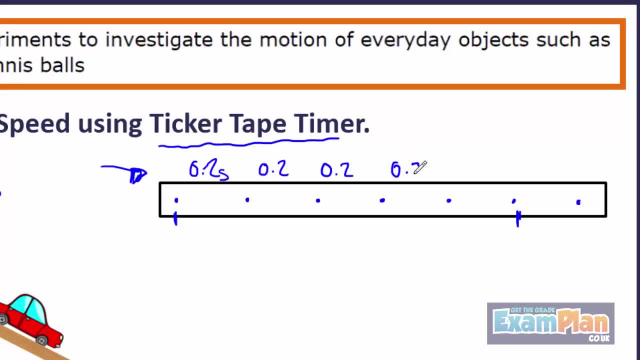 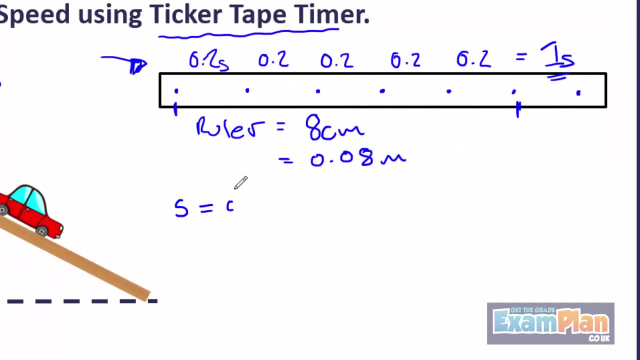 We know the interval between each dot is 0.2 seconds. so for 5 intervals we have a total time of 1 second. Measuring the distance between the dots with a ruler gives us a distance, so, for example, 8 centimetres or 0.08 metres. So the speed of the trolley is distance divided by time. 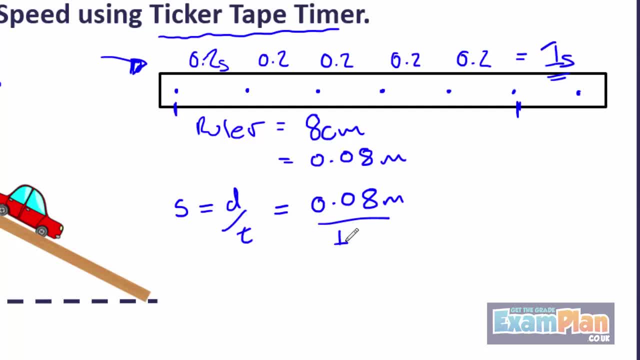 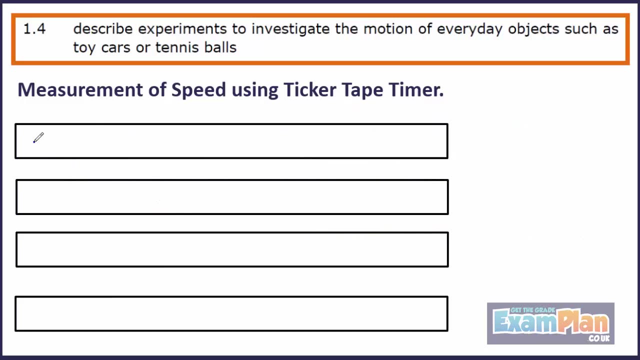 giving us a calculation of 0.08 metres divided by 1 second. So the speed is 0.08 metres per second. Different patterns of dots on the ticker tape tell us about the motion of the object. Constant spacing tells us the car is going at a constant speed. If the dots are further,